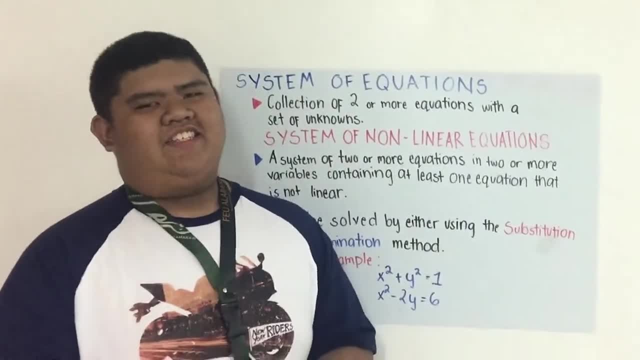 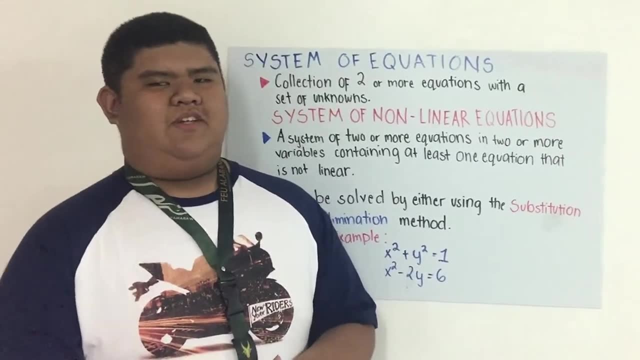 System of nonlinear equations. It is a system of two or more equations in two or more variables, containing at least one equation that is not linear. At least one of the variables has an exponent other than one where there is a product of variables in one of the equations. 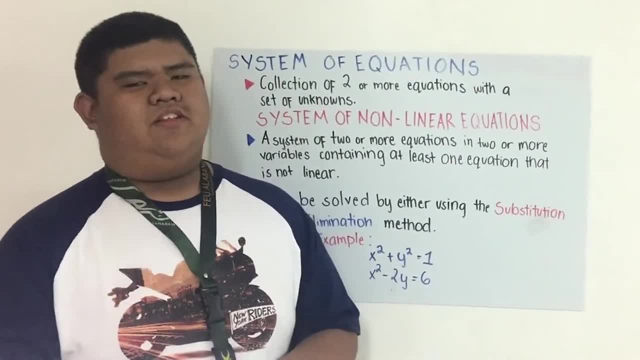 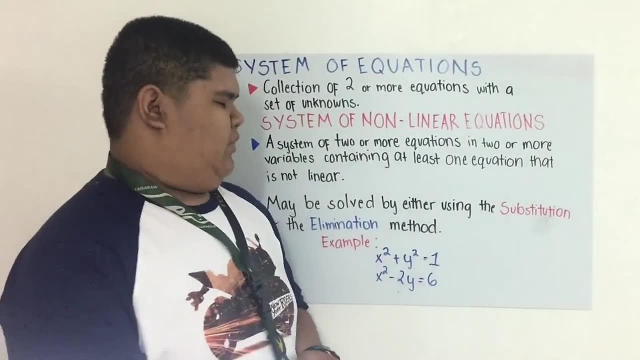 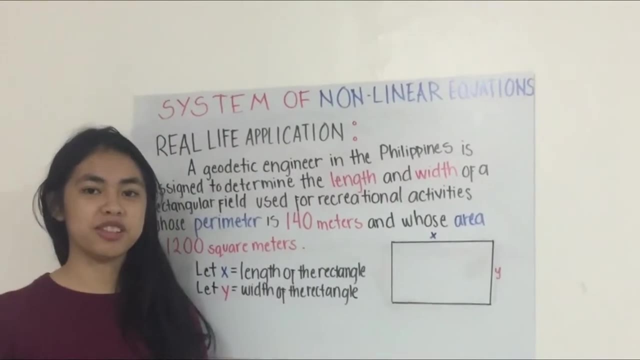 The system of nonlinear equations may be solved either using the substitution method or the elimination method. Here are examples of nonlinear equations: x squared plus y squared equals one. x squared minus two, y equals six. Systems of nonlinear equations are often represented in mathematical models used in engineering design. 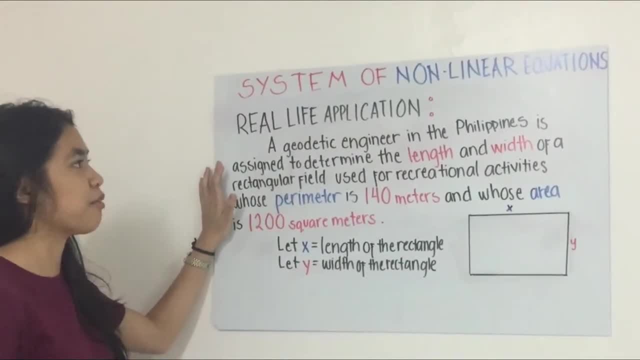 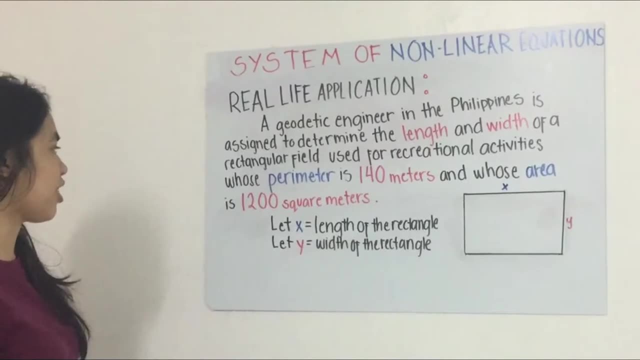 Here is one example of real life application of system of nonlinear equations. A geodetic engineer in the Philippines is assigned to determine the length and width of a system of nonlinear equations. This is the length and width of a rectangular field used for recreational activities. 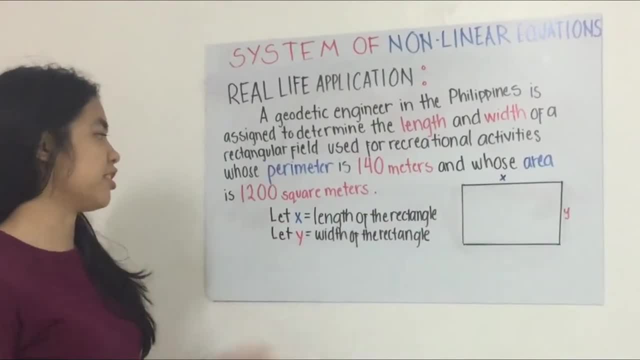 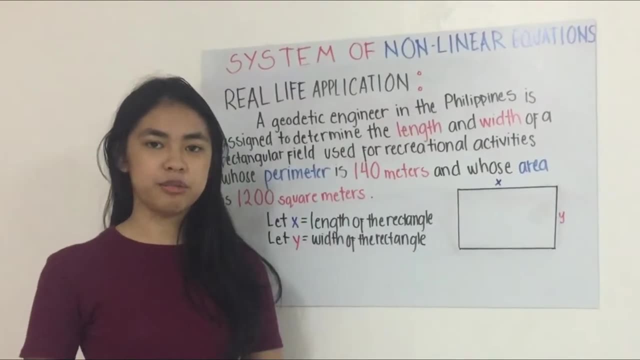 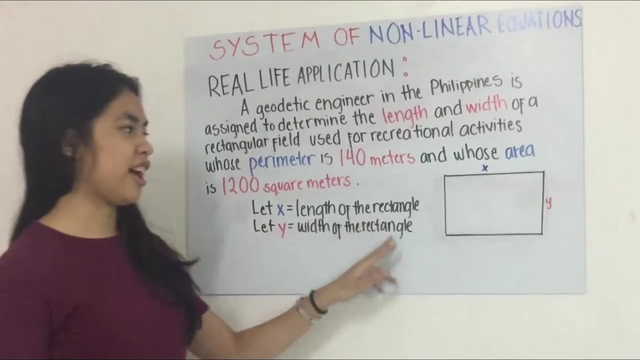 whose perimeter is 140 meters and whose area is 1200 square meters. So for our first step in solving this problem is to illustrate the problem and use variables to represent the unknown quantities. So let x be the length of the rectangle and let y be the width of the rectangle. 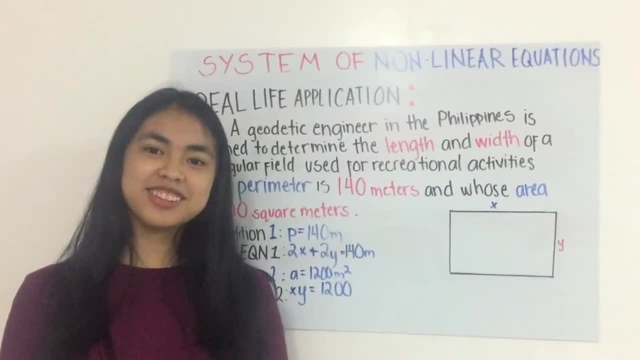 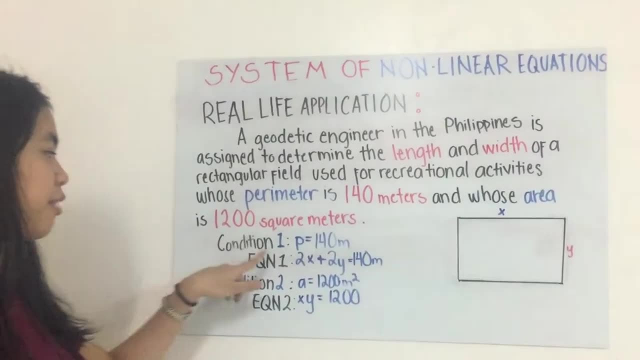 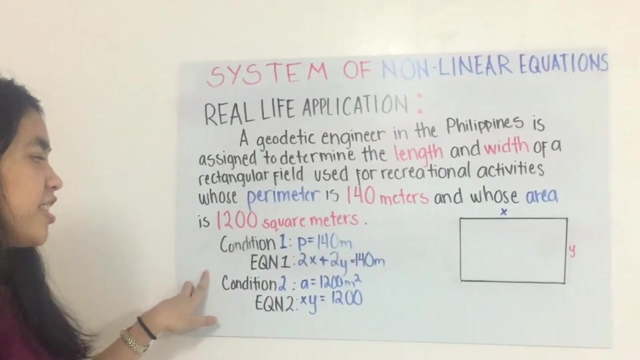 x squared. So for our second step is to write a system of equations that models the condition stated in the problem. So for the first condition, the perimeter is equal to 140 meters, And since we know that the formula for getting the perimeter of the rectangle 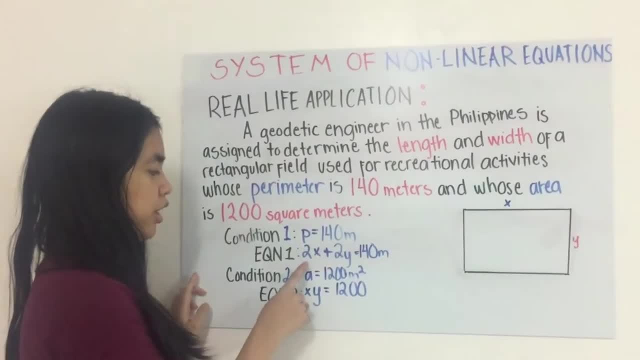 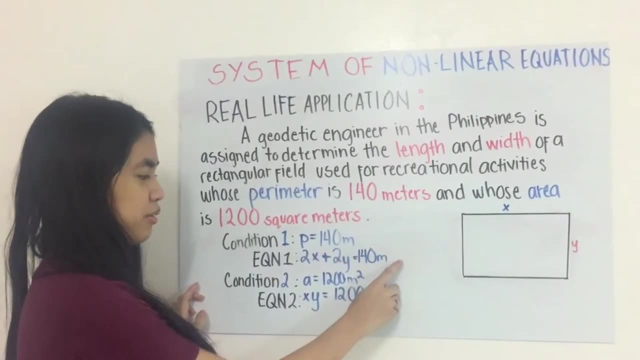 is P times length plus width. so our equation would be: 2x plus 2y is equal to 140 meters, which is derived from two times x plus y and equals to 140.. So for our next condition is that the area 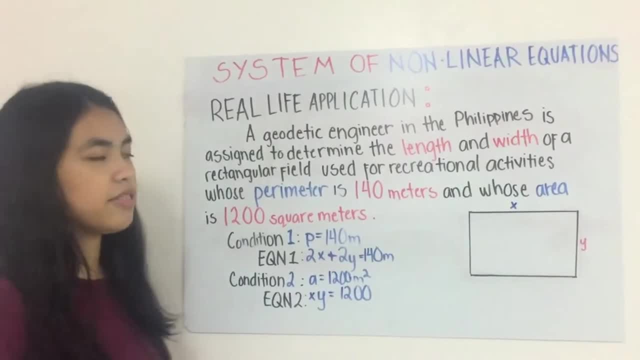 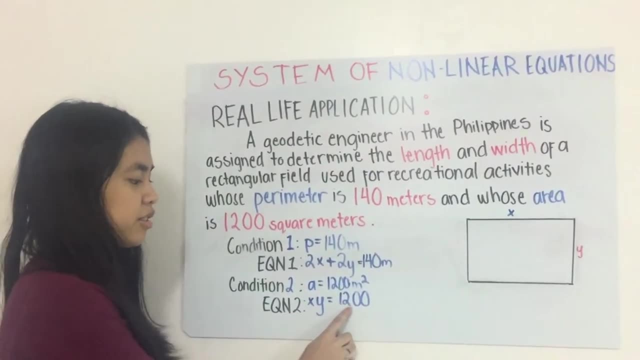 is equal to 1,200 meters squared, And since we know that the formula for getting the area of the rectangle is length times width, it would be: x times y equals to 1,200, which are represented by the length and width of the rectangle. 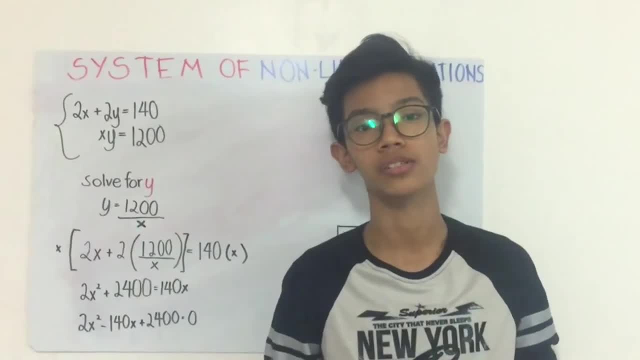 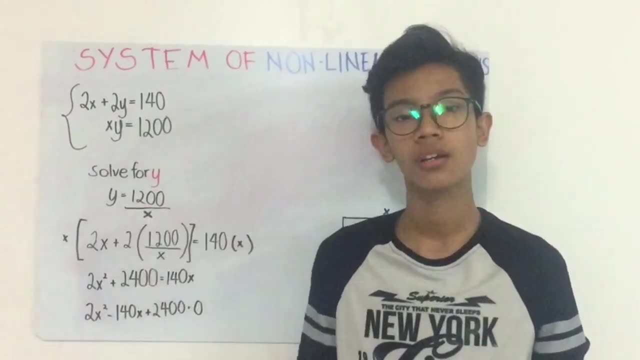 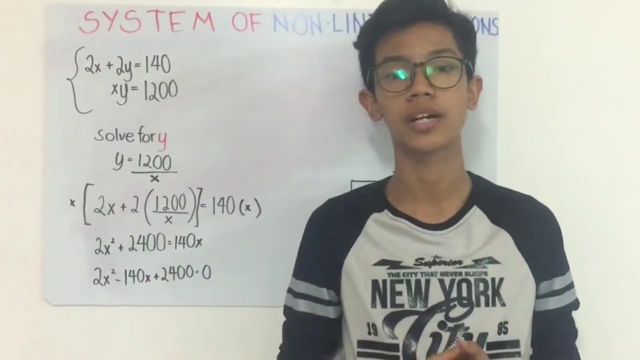 So for our third step is to solve the system of nonlinear equations. Use the substitution method in solving the system of equation. First we must solve for y. Substitute the value of y in equation one. to solve for x, Multiply both sides of the equation by x.